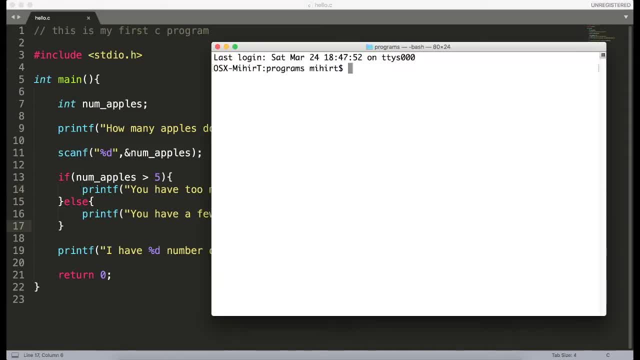 effort to make it as readable as you can. So let's try to compile and run this and let's see if this works. So we'll say gcc. so it compiles without any errors. Let's run it. How many apples do you have? 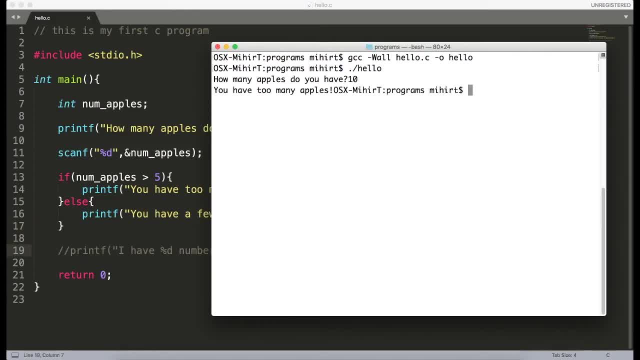 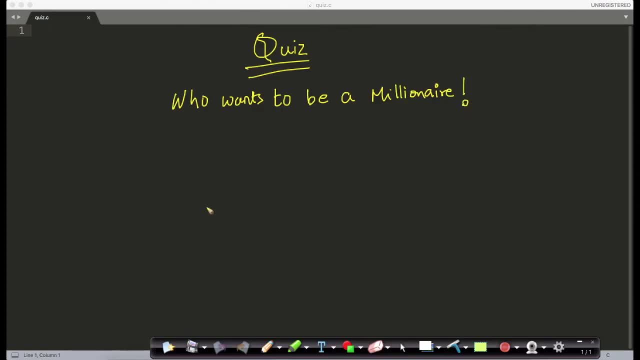 Let's say I say 10.. Now it does say you have too many apples. The only thing I don't like is you should have added a new line character over here. So with that you know enough of C language to do our first quiz, and your task is to create the game. who wants to be a millionaire? So as you, 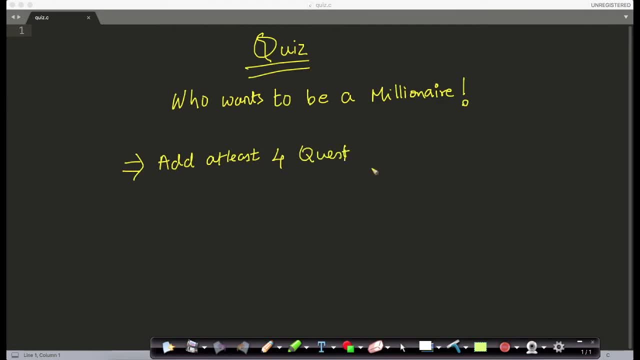 can see. essentially, we want you to create a quiz. We want you to have at least four questions. Each of the questions will have at least four options. If the user gives you a right answer, you should give him plus one point and minus one point for wrong answers And, in the end, your 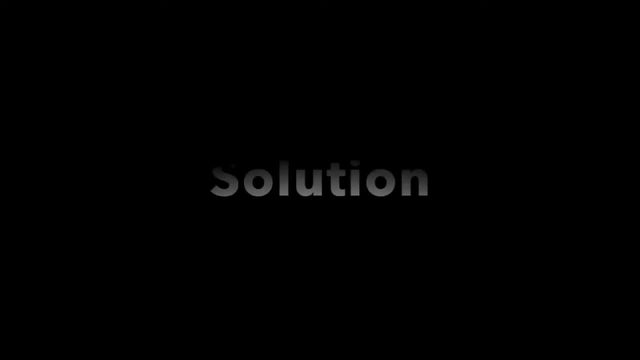 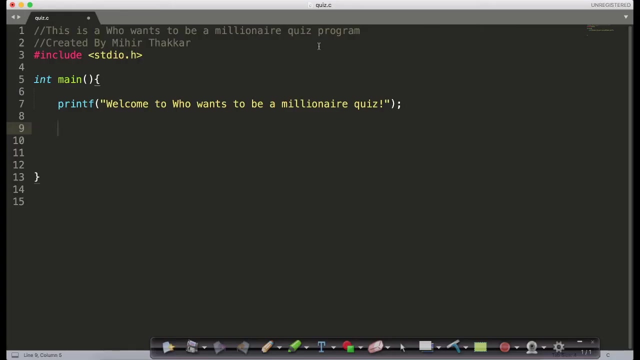 program should print out the user's final score. So this is how I would go about writing this program. First you set up your template and you do all the rest of the work. Then you go to the regular stuff that you do, You include the stdioh file and then we welcome our user to the game. 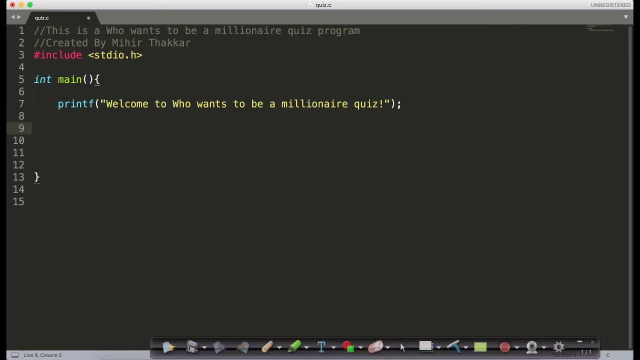 Next, let's go ahead and write our first question, So we'll say printf: who is the president of United States? Then let's give users four options. And now we want to wait for the users to give us their input And, as we saw in our previous videos, the way you would take input from the user is by 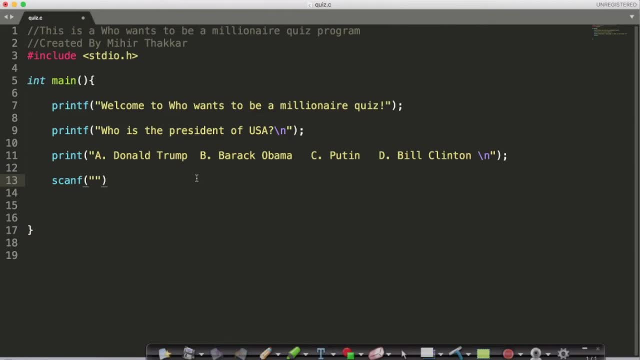 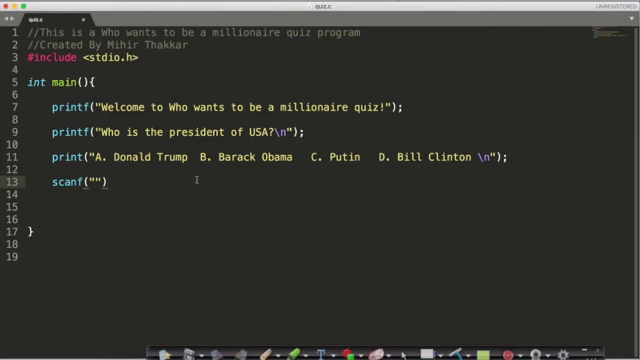 using the scanf statement. So in the previous video we were talking about how to input the percentile D. So in the previous videos we have seen that to scan an integer we use a percentile D. We want to scan if the user is typing in option A, B, C or D. So what should we write over here? 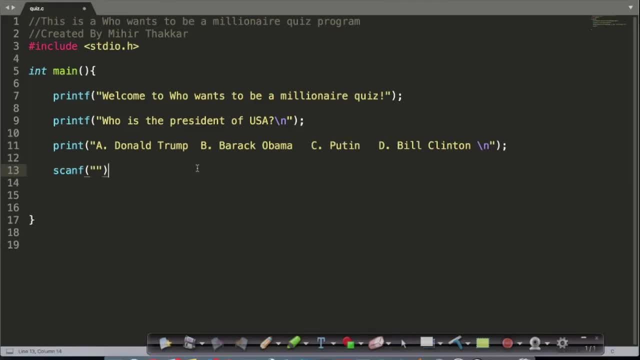 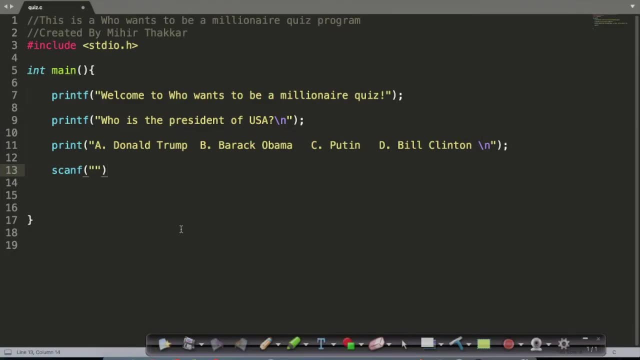 to scan your character. Well, in this course, I'm not always going to tell you what you should be using, And in such situations, your best friend is going to be Google. So if I were you, I would go to Google and say percentile D. 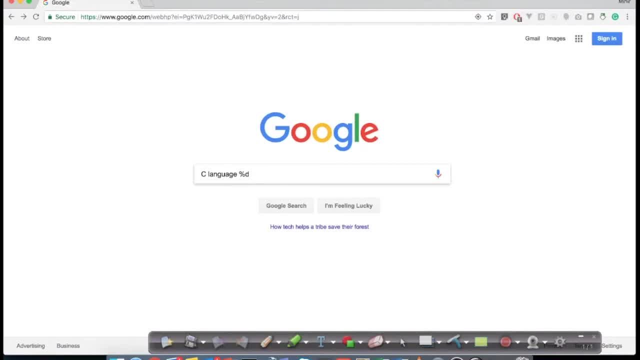 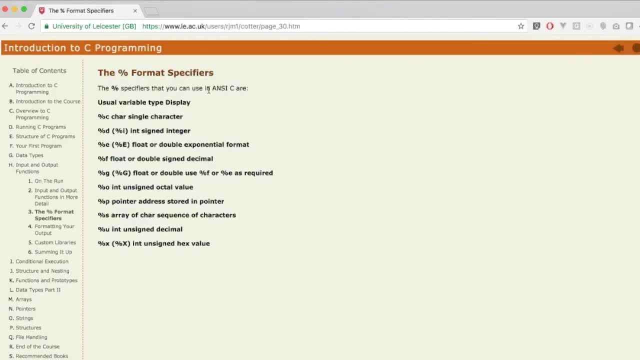 So I would say C language first. Say percentile D is integer, Let's see what we get. This concept seems to be called format specifiers. So the percentile is the format specifiers. The percentile specifiers that you can use in C are percentile C for character. 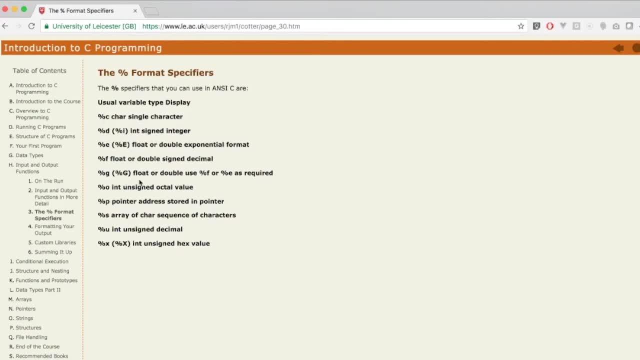 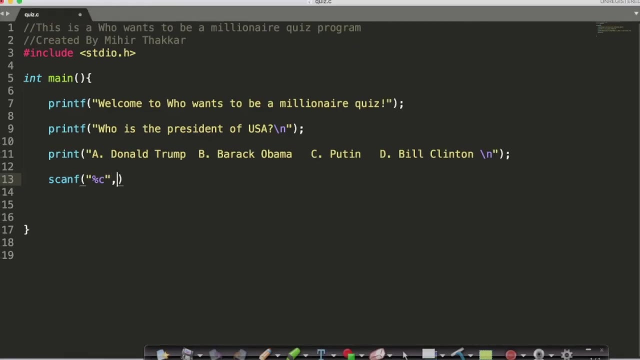 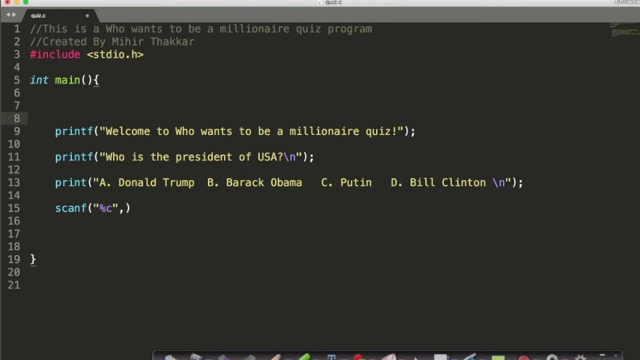 percentile D for integer and so on, And what we want is to scan a character, So we'll use the percentile C. Let's go back to our program and say percentile C, So we don't have a location to store the answer. So let's go ahead and write a location where we'll store our answers. 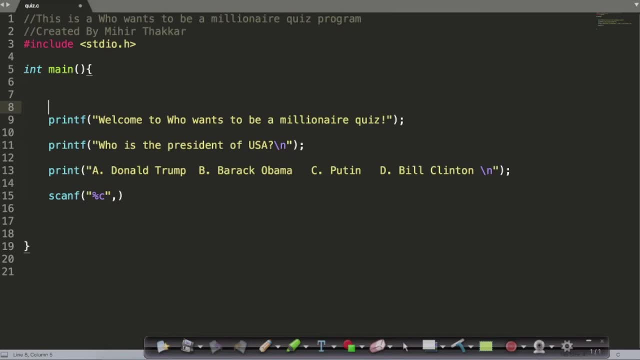 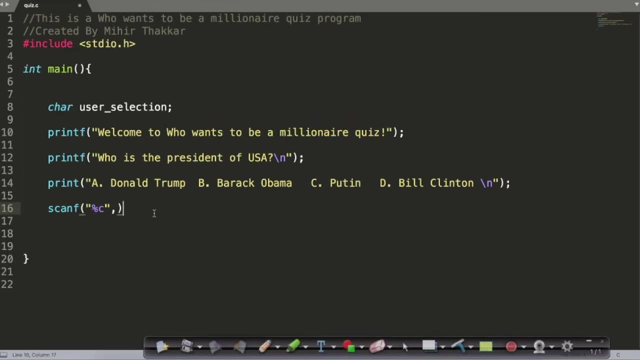 So what should its type be? The way you define characters in C language is by using the keyword care. So it's a care. Let's say user selection And we'll store the answer. So we'll store the user's answer at address of user selection. 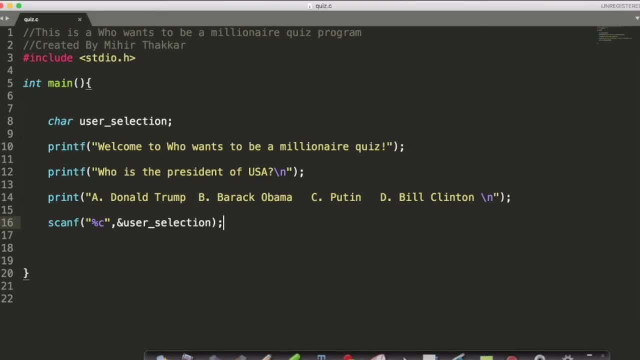 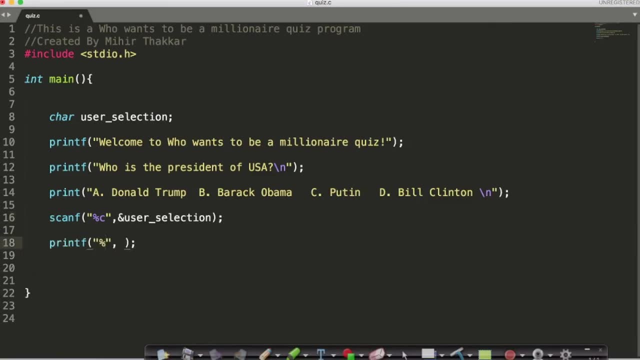 Right. So as soon as I reach this point, if I were you, I would first print it out to the screen and see if I have done this part correctly before moving ahead. So let's just print this user selection out. So let's say: user selected: percentile C: user selection: 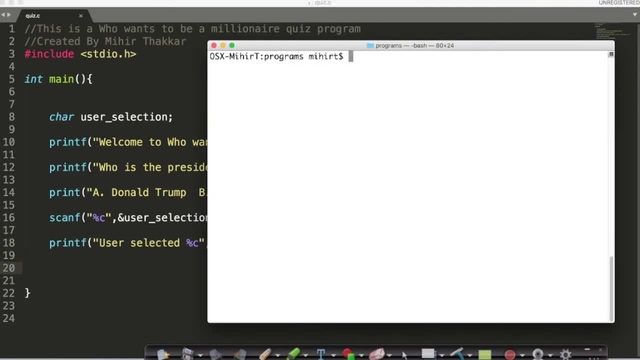 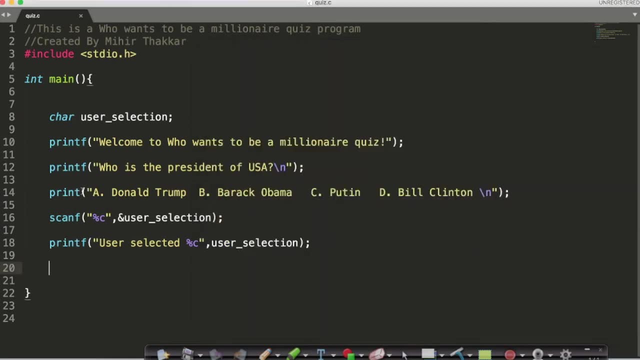 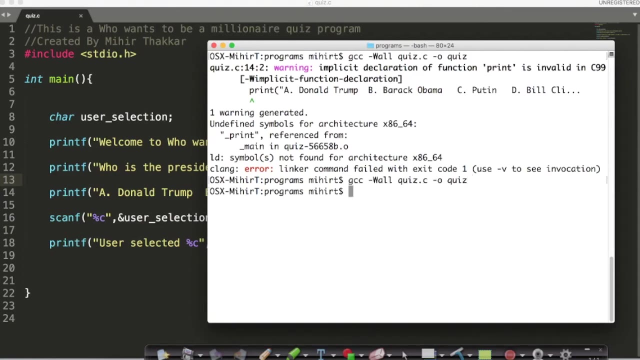 Right. So let's first clear the screen, Then we'll say: Let's compile this. I mean there is an error, So we need to say printf. So now let's try that again. It compiles without any errors, So it means that we are OK. 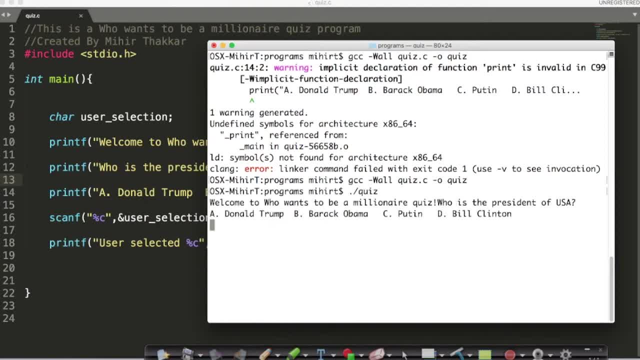 Let's try to run this. So the first two print statements went correctly. Next it's asking us to give an input. Let's say we said A. It says user selected A. So I think our program is doing fine Until here. 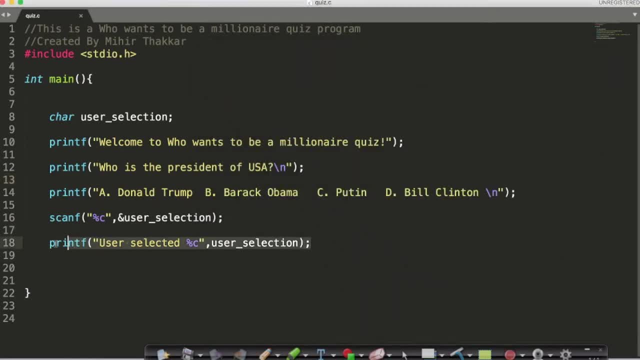 Let's go back to our program. We don't need this statement. We were just checking if we are correct until here. Now we want to check if the answer was correct. So we'll say: if user selection is equal to, equal to A,